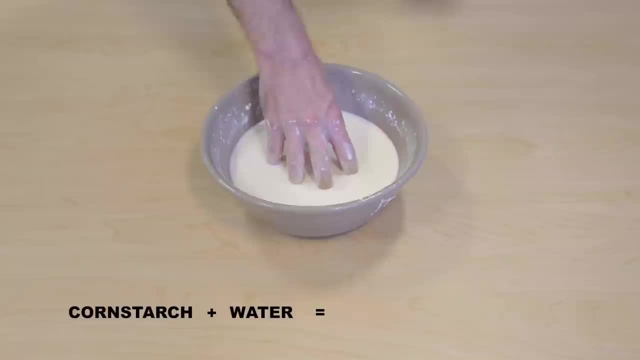 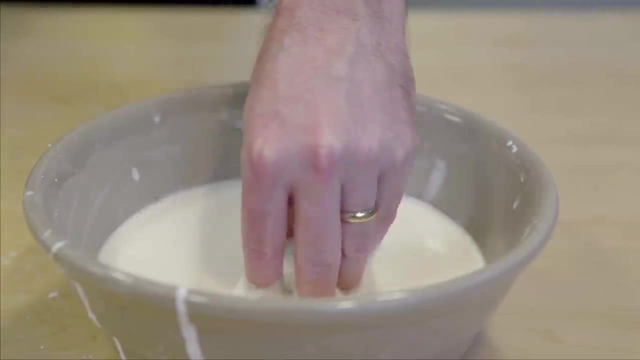 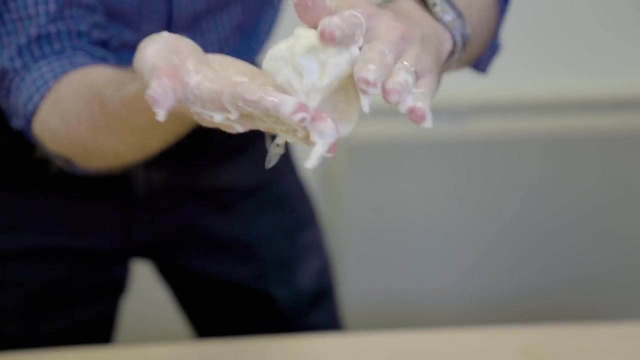 When you mix cornstarch in water, weird things happen. Swish it gently in a bowl and the mixture moves like a liquid. Squeeze it and it starts to feel like paste. Roll it between your hands and it solidifies into a rubbery ball. until you try to hold that ball in the 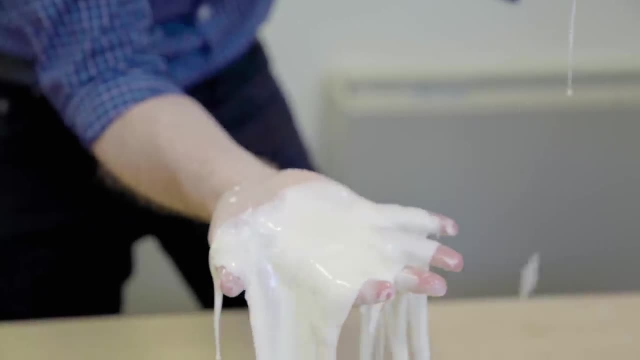 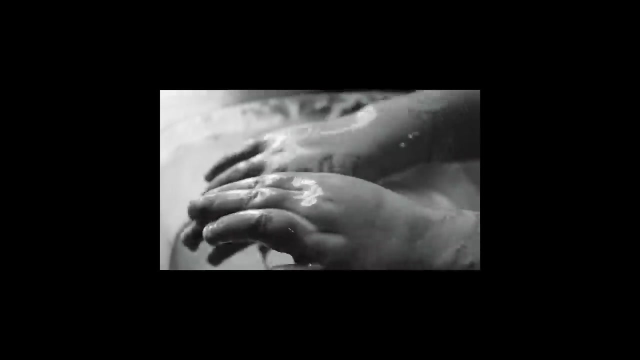 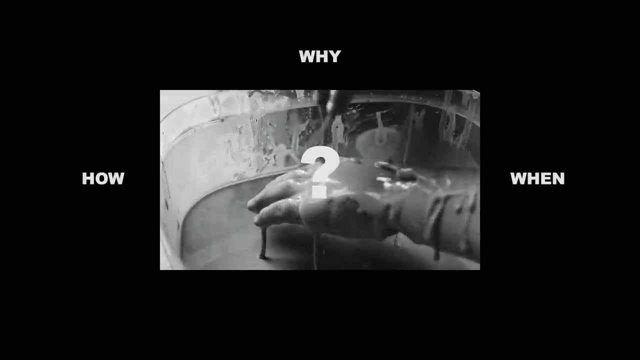 palm of your hand and it loses its structure and dribbles away. To many who have played with this material, perhaps as children, its strange behavior is nothing new, But understanding exactly how, why and when this material will act a certain way has always been rather unpredictable. 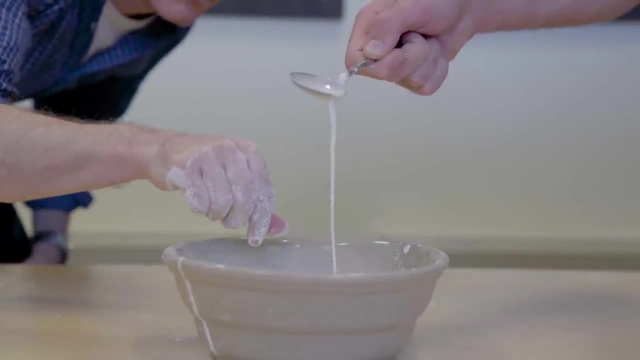 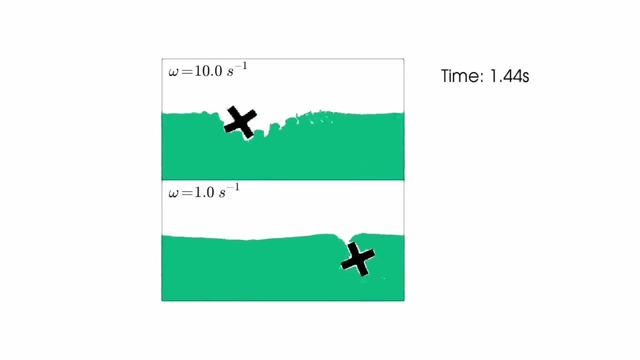 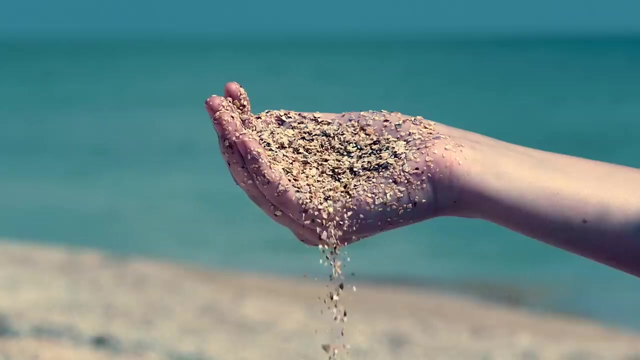 But now a team of MIT engineers have developed a mathematical model that can accurately predict this material's behavior under various conditions. A single particle of cornstarch is about 1 to 10 microns wide and about 100 times smaller than a grain of sand. It turns out that particles at 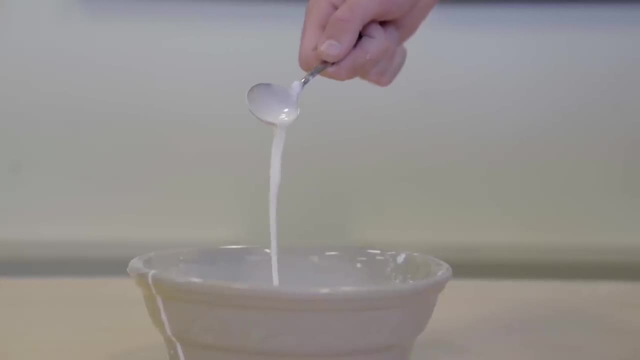 such a small scale experience effects. The larger particles do not. Because cornstarch particles are so small, they can be influenced by temperature and by electric charges that build up between them, which causes them to slightly repel against each other. So as long as you move slowly, the grains will repel and slide past each. 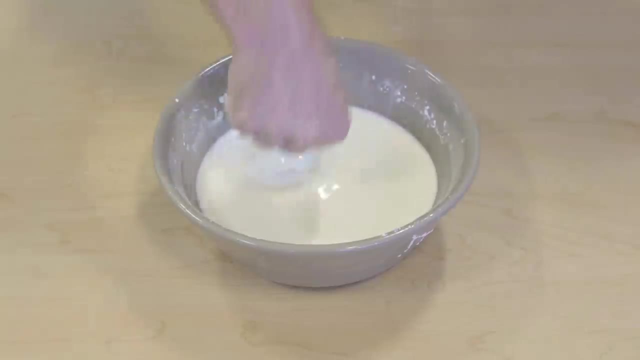 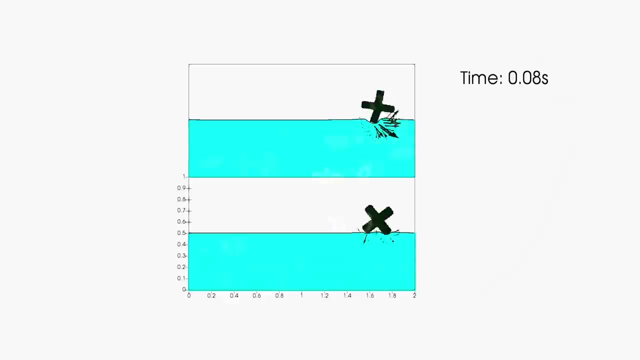 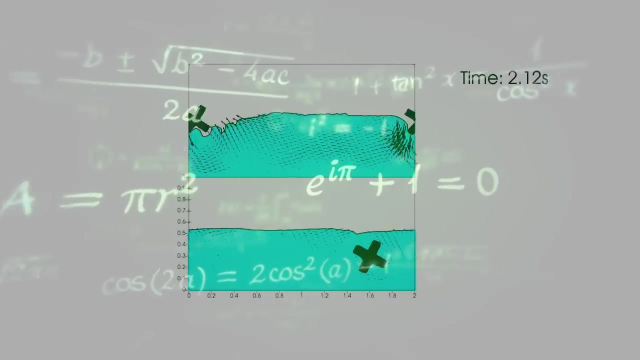 other like a fluid. But if you do anything too fast, you'll overcome that repulsion. The particles will touch, there will be friction and it will act as a solid. The researchers incorporated equations in the model to describe the effects of particle repulsion and the speed at which the material is. 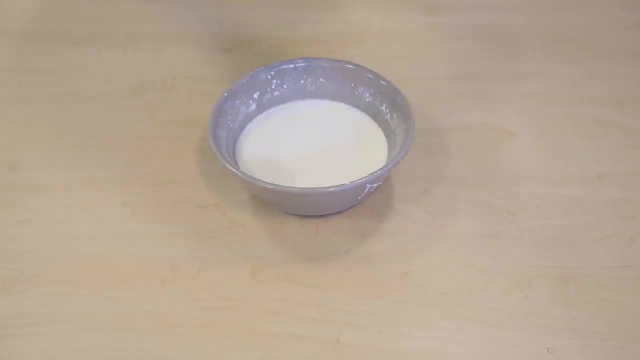 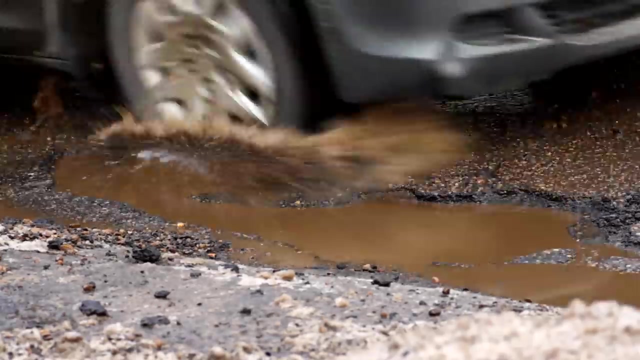 deformed to predict whether it would behave as a solid or a liquid under various scenarios. The researchers say the new model can be used to explore how various ultra-fine particle solutions, such as cornstarch and water, behave when put to use as, for instance, fillings. for potholes or bulletproof vests. 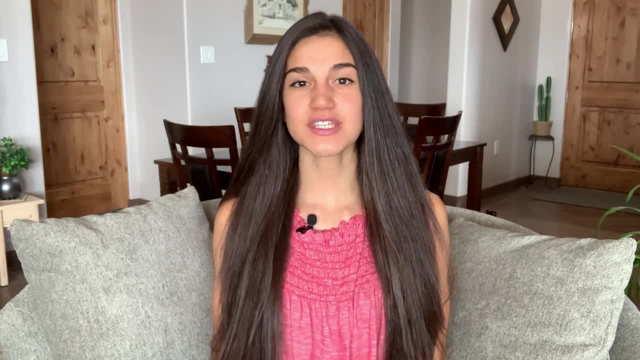 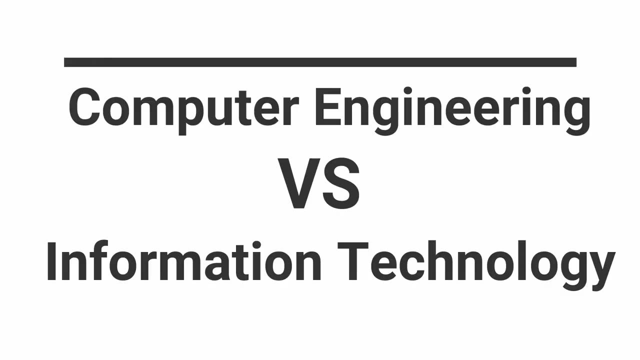 Hello everyone, welcome back to my channel. In this video, I'm going to talk about the differences between computer engineering and IT, So let's get started, All right. so I've been getting a lot of questions as to what is the difference between computer.